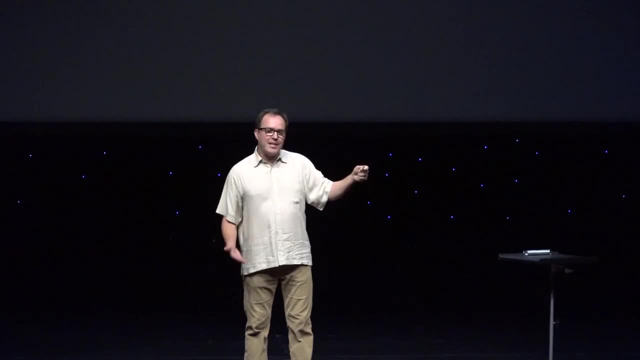 about the mid-1500s. In the early 1600s, Galileo became the first person that we know of to really investigate the physical properties of a pendulum, And he was able to come to some pretty dramatic conclusions, Like, for example, Galileo was able to show that the period of the pendulum 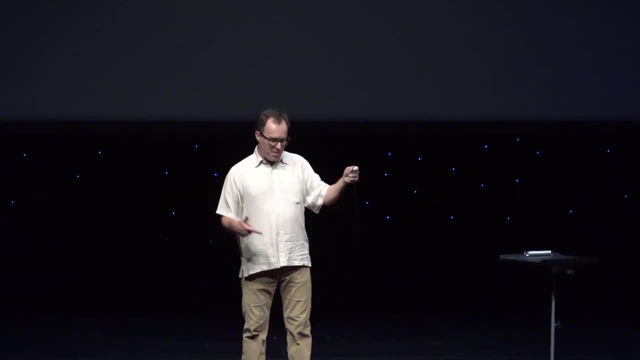 which takes to go through one complete cycle is independent of the mass that is at the end of the pendulum. So if I was to replace this mass with something a little bit bigger, a little bit smaller, we would see that this motion would be about the same. The work of Galileo was extended. 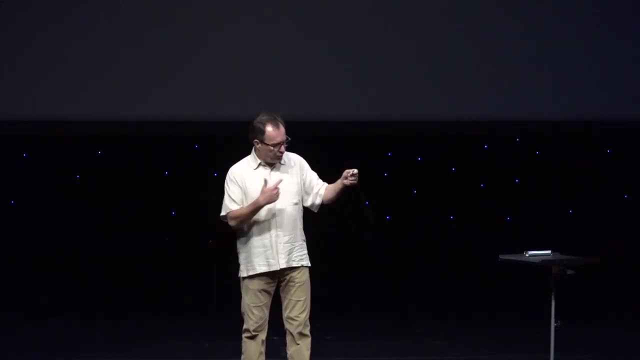 about 100 years later, by Sir Isaac Newton, who was able to fully describe the motion of the pendulum, showing that its motion is completely determined by the length of the pendulum and the gravitational pull of the pendulum. So if I were to replace this mass with something a little bit bigger, 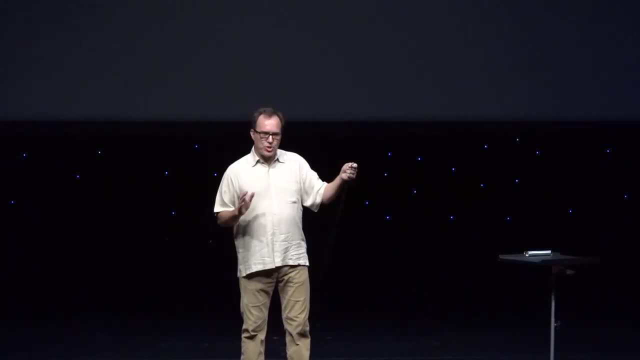 it would be about the length of the earth. In fact, Newton was able to show with the computations involving a pendulum that the earth is not a perfect sphere. It's pretty close to perfect, but it turns out that it's squished a little bit on the top and bottom and has a bit of a bulge going around. 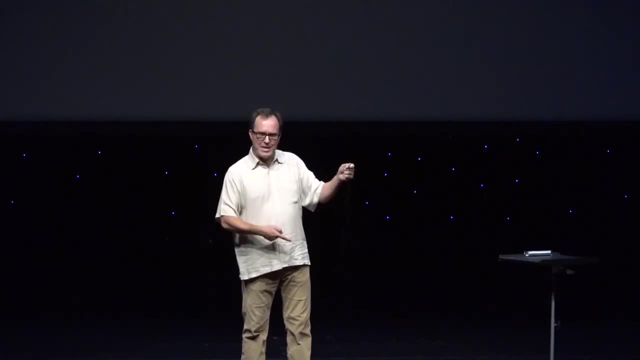 the middle, And Newton was able to show that with one of these, which I find absolutely amazing. Now, under ideal circumstances, this pendulum would swing back and forth like this forever, But as I stand here on the Smith Center stage, these are not ideal circumstances. I should be holding my hand. 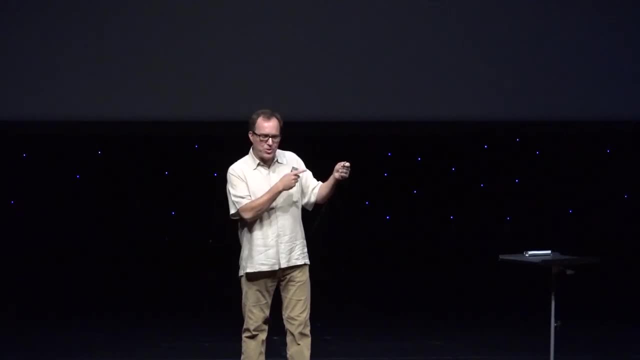 perfectly still. I'm doing the best that I can, but I'm sure that there's a little bit of movement there. More importantly, there's a bit of air resistance that is acting against the motion of the pendulum as it's swinging back and forth, And if we waited long enough, we would see this. 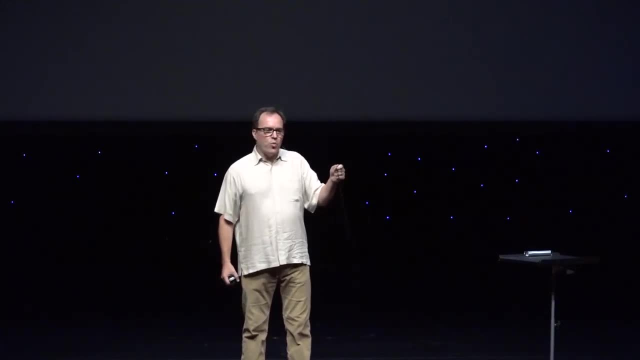 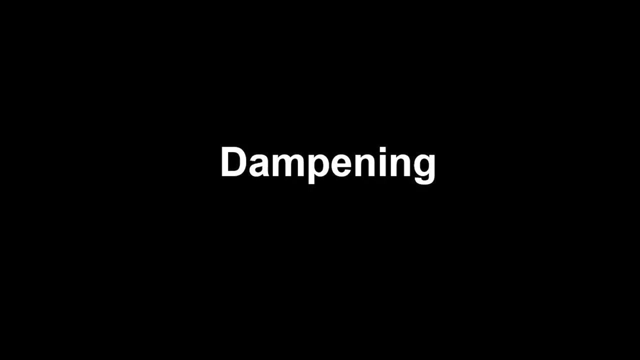 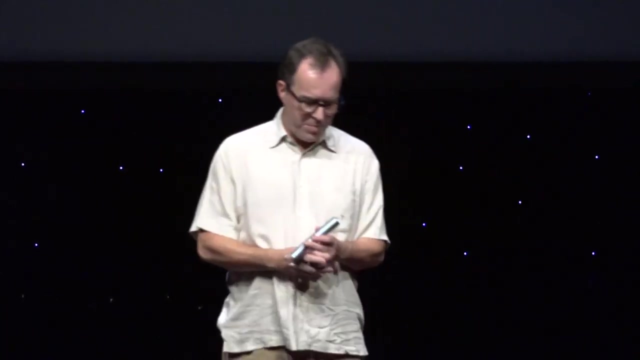 pendulum eventually slow and come to a stop. When you have a mechanical system that is oscillating but the magnitude of the oscillations are decreasing. that is what we call dampening And dampening understanding. dampening involves looking at imaginary numbers. Now why might you be interested in dampening? Well, I also brought with me a 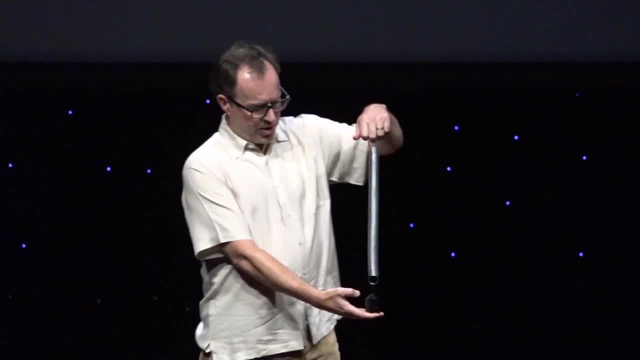 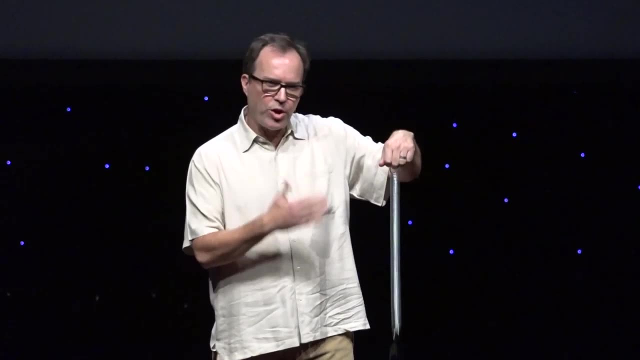 spring. I'm going to attach the same mass to it. let it stretch out to its equilibrium position. give it a little bit of a push and it's going to oscillate. Yes, these oscillations are vertical. while the pendulum was swinging back and forth. 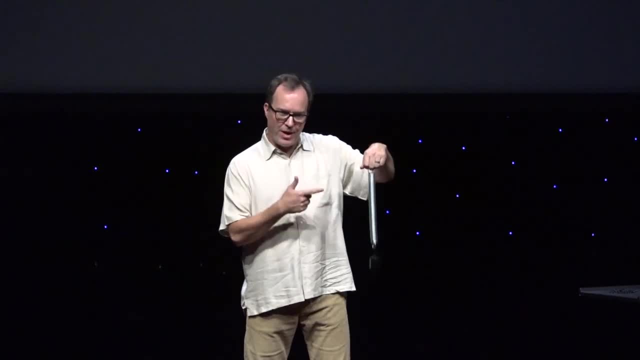 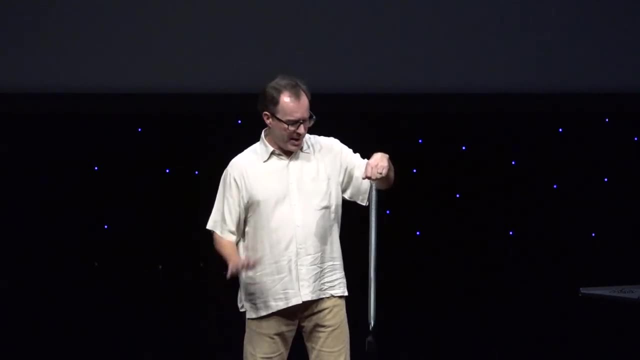 I am more likely to get a victory of probability than never have I in my life. This pendulum is the average that the equations that describe this kind of oscillating motion and the equations that describe the pendulum swinging back and forth are pretty much pretty close to the same equations. They have a lot of similarities. It also turns 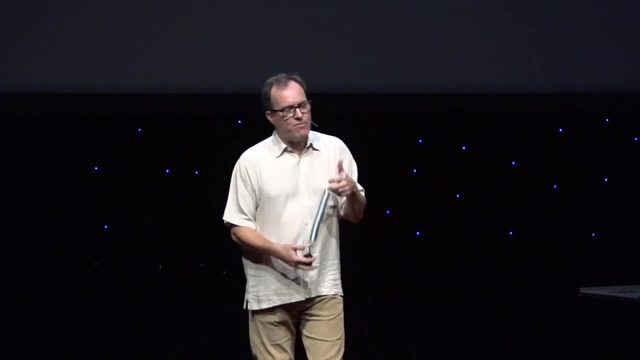 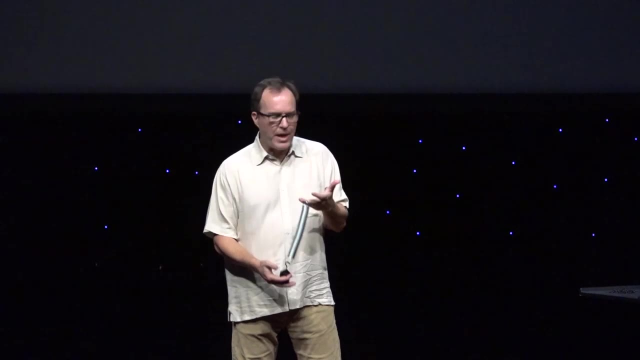 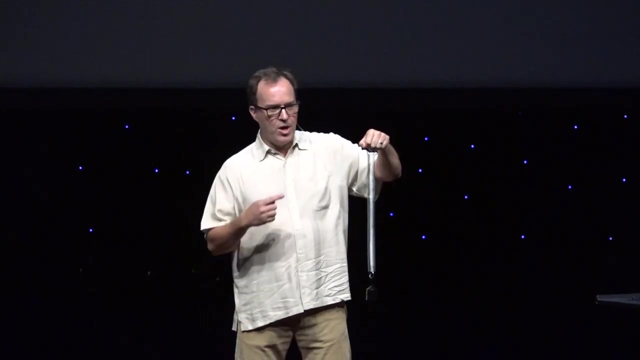 out that a spring mass system such as this is a very simplified but reasonably accurate model for the suspension system in your car. When you are driving along and you have a smooth ride, it's equivalent to my spring mass system being here in the equilibrium position When you go over a bump. that bump sets. 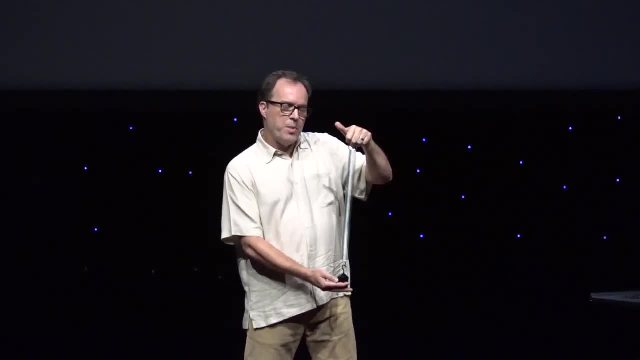 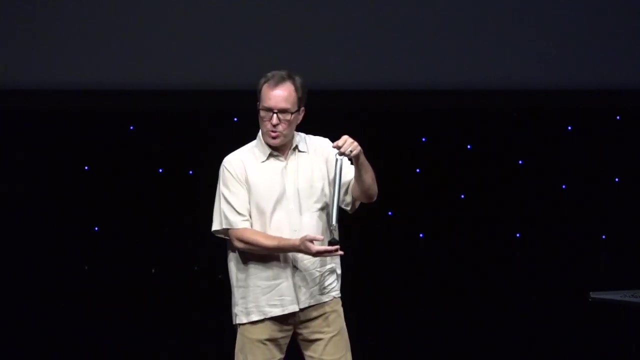 the suspension system into an oscillating motion, but the dampening that's built into the system quickly- hopefully gently- bring you back to the equilibrium position. The oscillations allow the suspension system to absorb the bump, while the dampening quickly bring you back to a smooth ride, So like 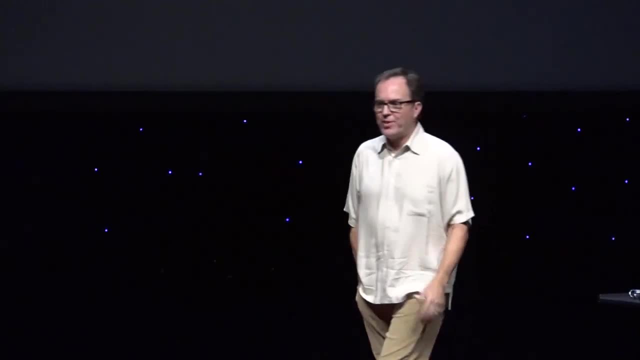 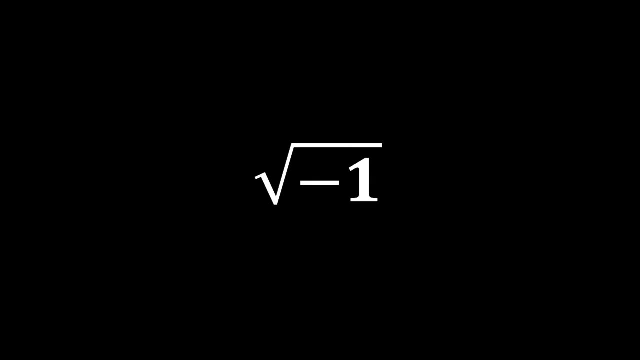 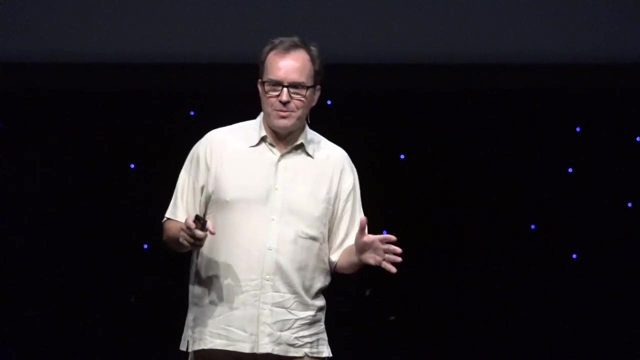 I said, when you are studying the math and physics involved in dampening, you very quickly come across needing to know what is the square root of negative one. And while today's algebra students know exactly what to do with this, this is a question that stumped mathematicians for centuries. Let's talk. 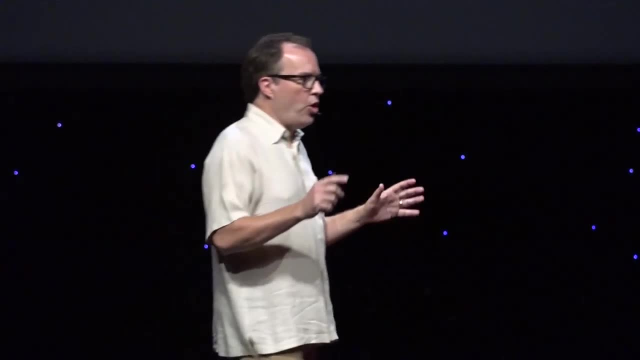 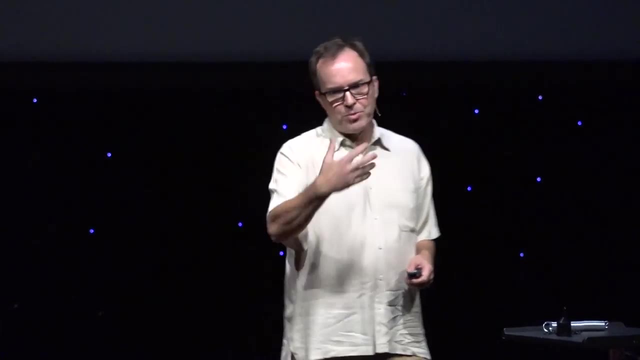 a little bit about why We come across numbers all day, every day in our lives. Maybe I ask you: how far away do you live from Ohlone College? You're gonna respond to me with a number. Maybe it's the number of miles between. 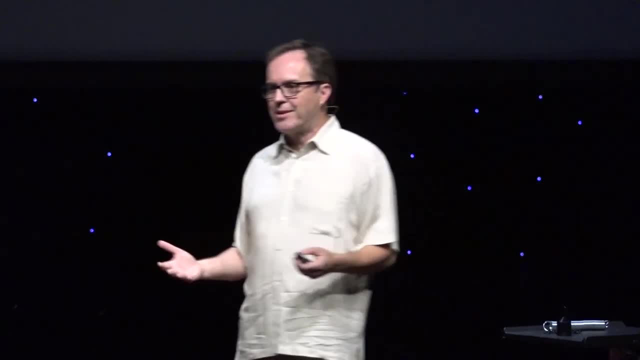 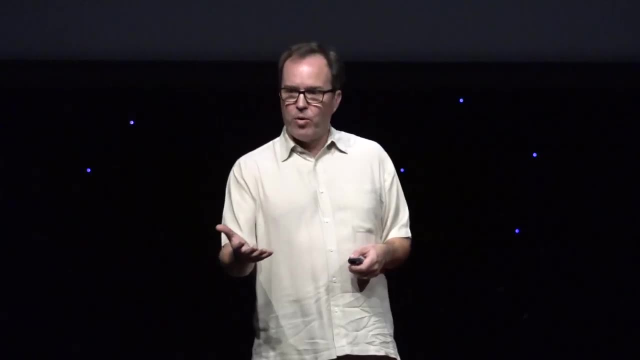 where we are and where you live. Maybe it's the number of minutes that it's going to take for you to get home after tonight's events. But you're gonna respond to me with a number. Maybe I ask you how old you are. You're gonna give me. 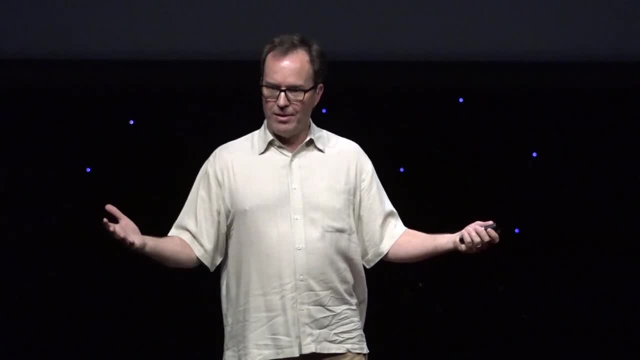 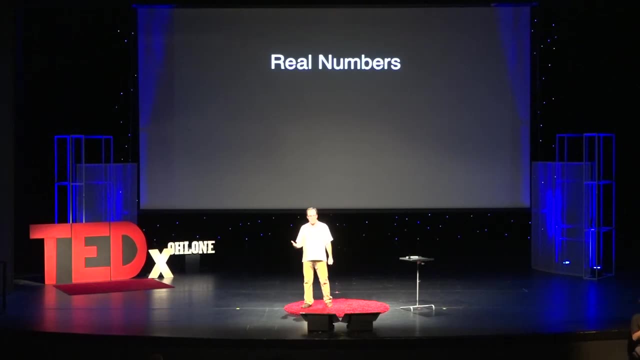 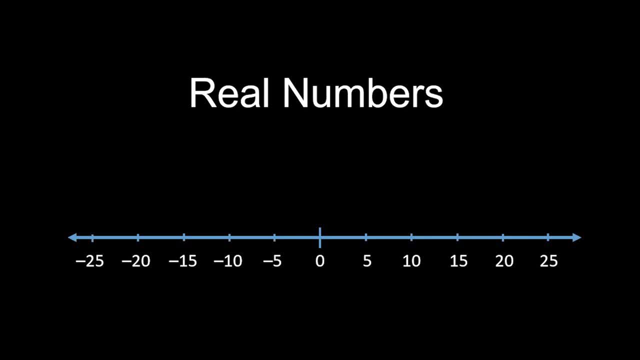 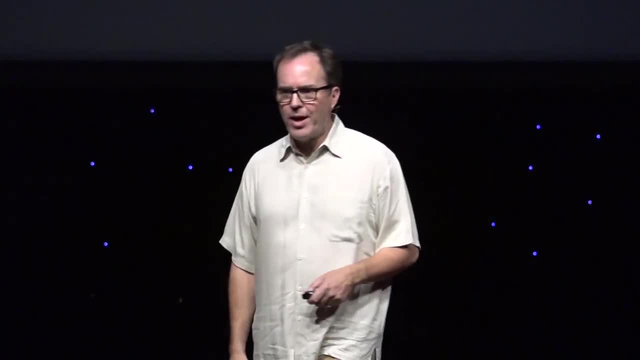 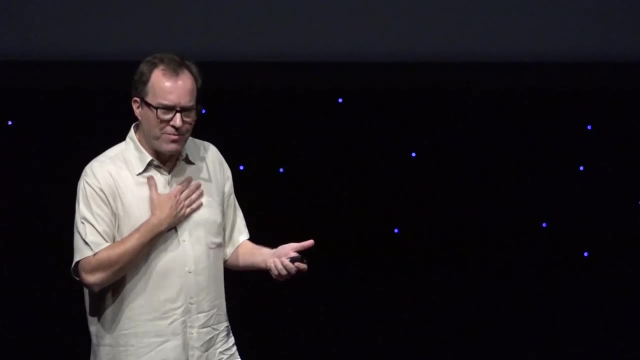 Maybe. I ask you how much money is in your checking account and unfortunately, the answer is negative $18.. That is something that I can plot on the number line and so therefore it is a real number. By the way, if you do have negative $18 in your checking account, I feel your pain. I have. 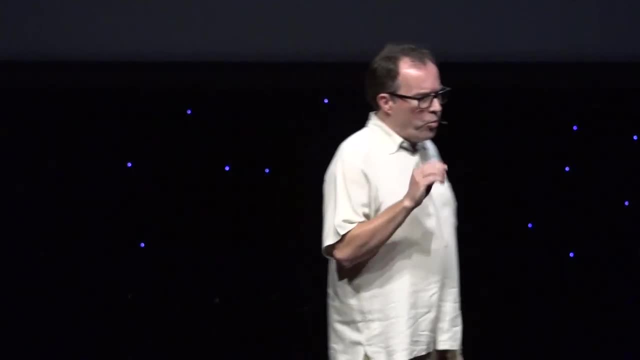 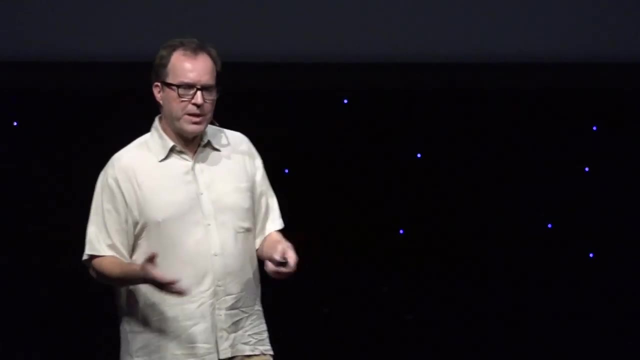 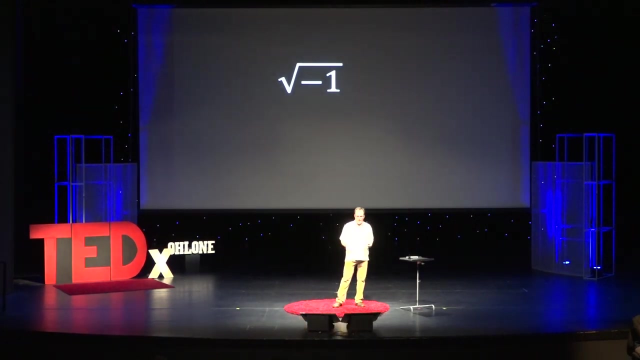 absolutely been there. Okay, so one of the properties of real numbers is that every real number- positive and negative- when it is squared becomes positive. We are looking for the square root of negative 1. Whatever that number is going to be, it has to be the case that when we square that number, we would end 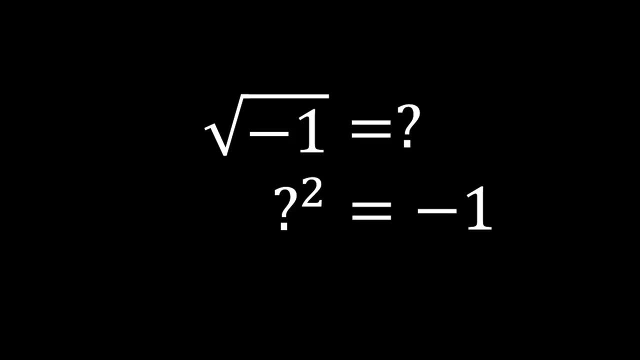 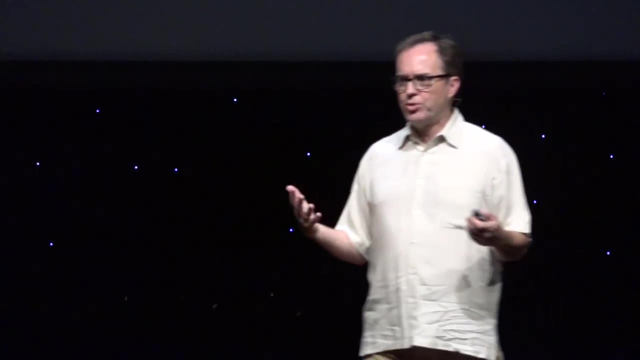 up with negative 1.. Since no real numbers have that property, the square root of negative 1 cannot be a real number. This became a stopping point in doing mathematics for centuries. If you were working and you came across the square root of negative 1, it was assumed that there was no solution and therefore the 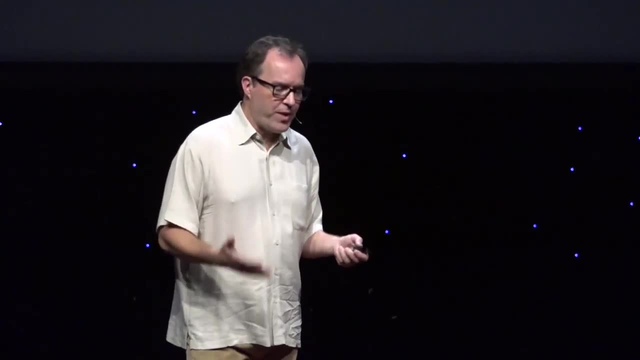 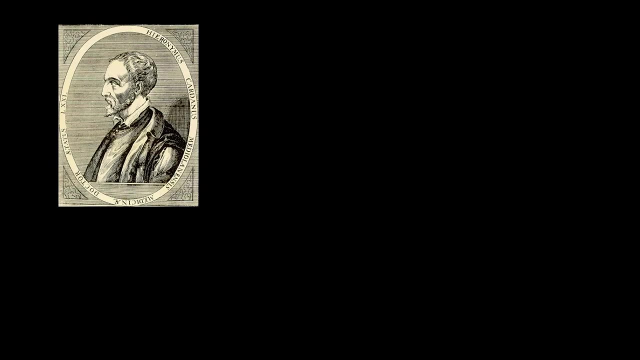 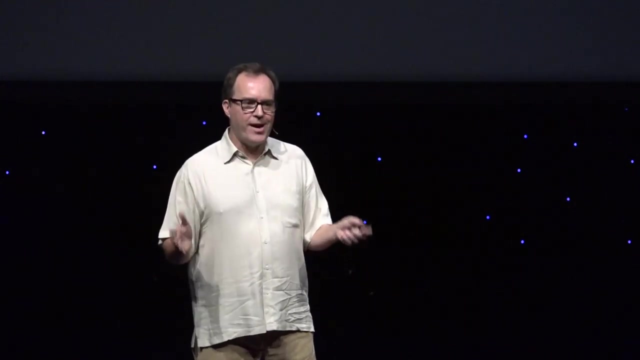 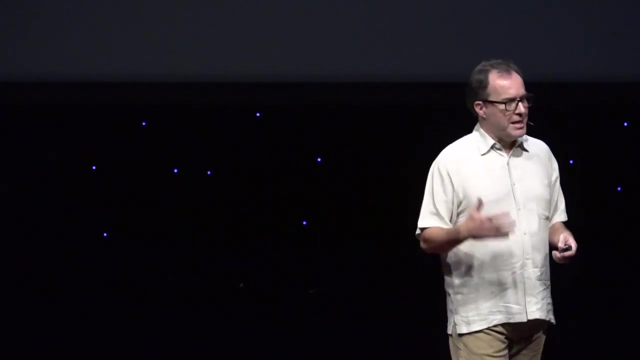 problem stopped. It wasn't until 1545 when an Italian mathematician named Guillermo Cardeno came up with an extraordinary idea. He made up a new number. He literally broke free and defined the undefined. Now, the number that he made up is what we now know to be the imaginary number i. He did not. 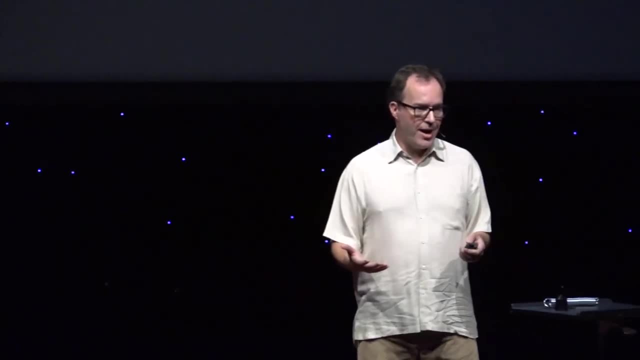 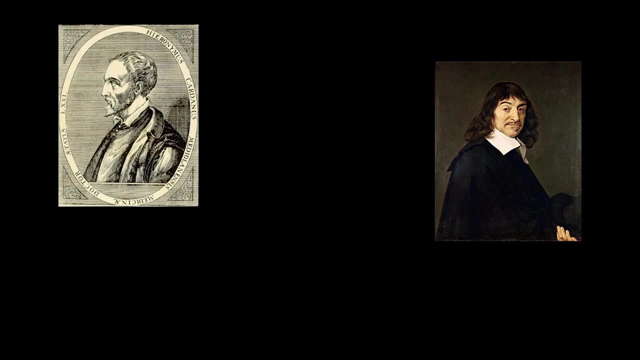 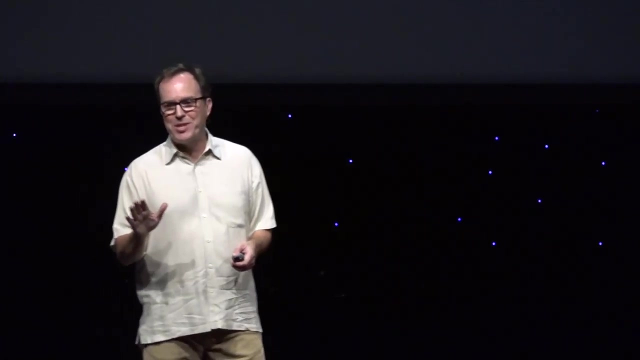 call this an imaginary number, nor did he use the notation i. It wasn't until almost a hundred years later that the mathematician Rene Descartes started referring to these numbers as being imaginary, And, interestingly enough, he did it in somewhat of a derogatory way. He was not happy about these numbers. 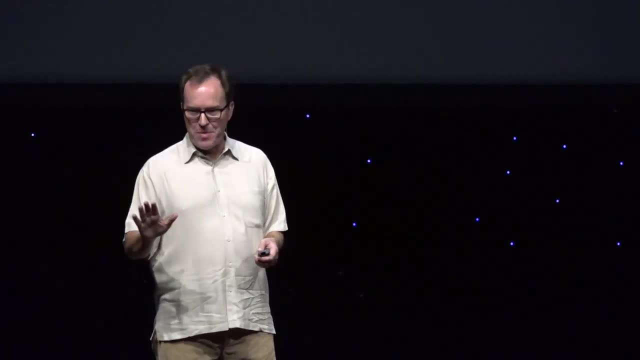 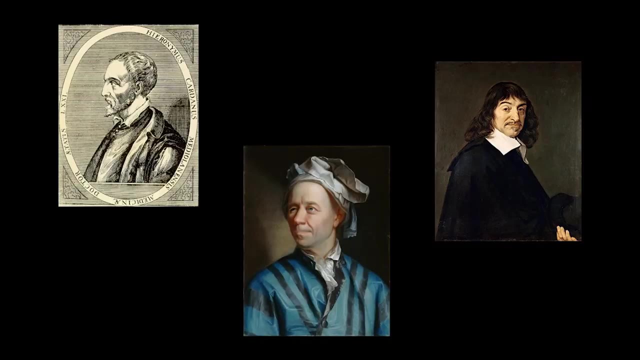 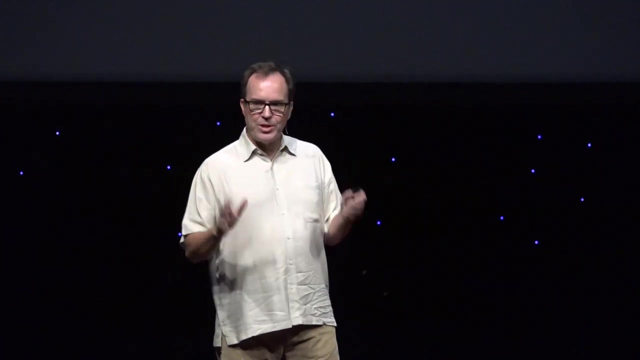 needing to exist and did not like them and started calling them imaginary. And then it was almost another hundred years when the great mathematician Leonard Euler started referring to them with the notation i that we are familiar with today. Worth noting that Leonard Euler is absolutely the most prolific mathematician of all time. Now we have this new 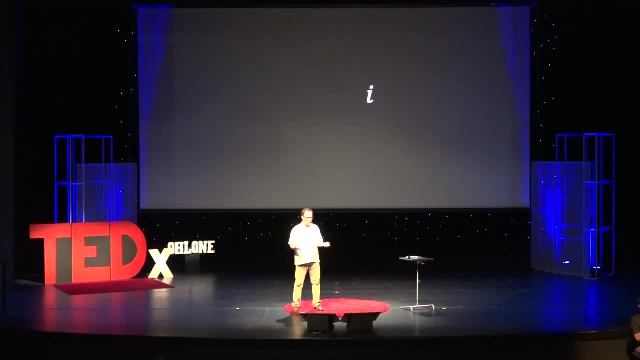 number. It's an imaginary number. It's denoted by the number i. If you take the imaginary number i and you multiply it by a real number, then we still consider that to be an imaginary number. If you add a real number to that, then you get. 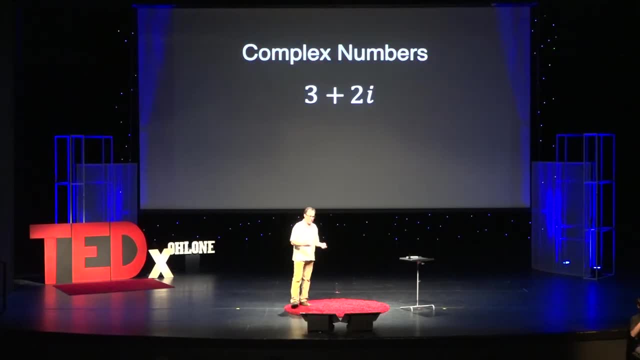 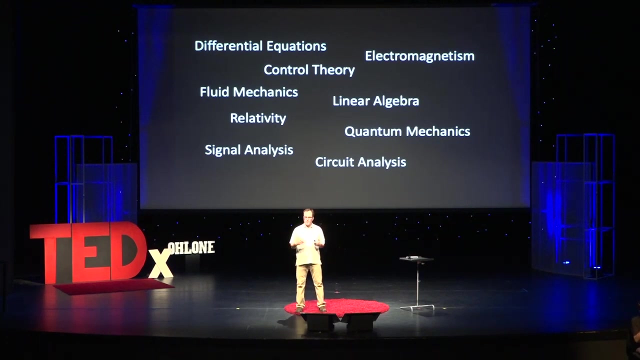 what we mathematicians call a complex number, And complex numbers have applications in all sorts of mathematics, Math, physics, engineering and other sciences. All of these are topics where, if you are going to study them, you need to have a basic understanding of complex. 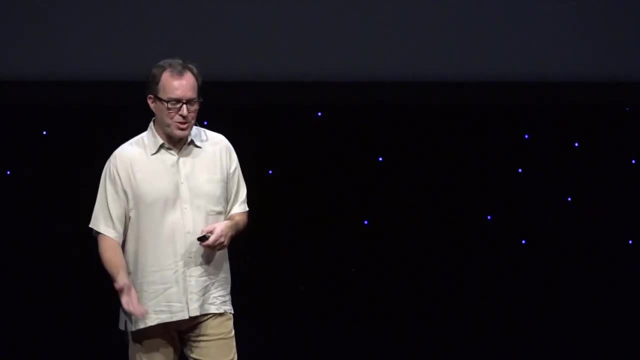 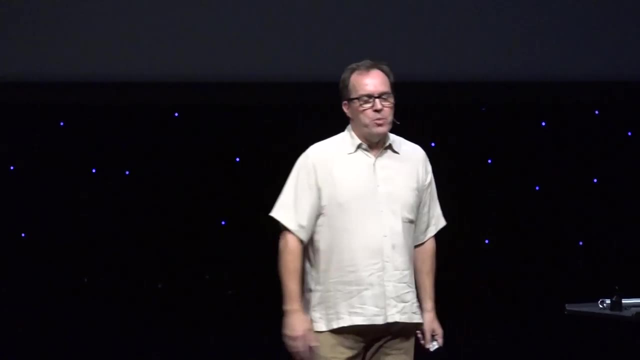 and imaginary numbers. The next thing that I would like to show you is called Euler's identity. Now, we just saw Euler. He was the one who came up with the notation for i, Most prolific mathematician of all time. there is a. 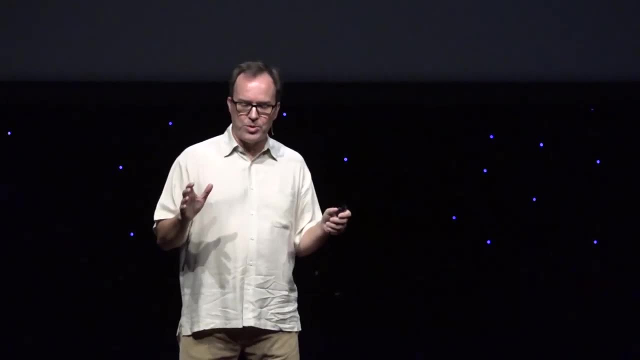 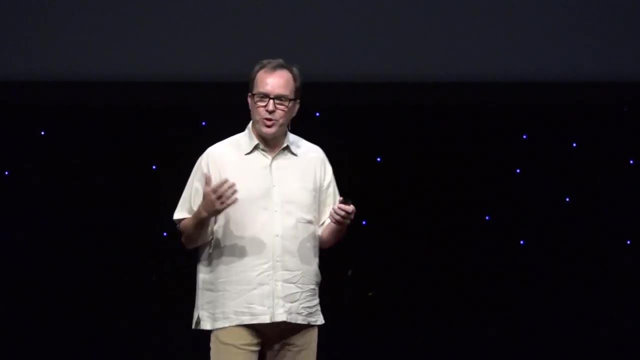 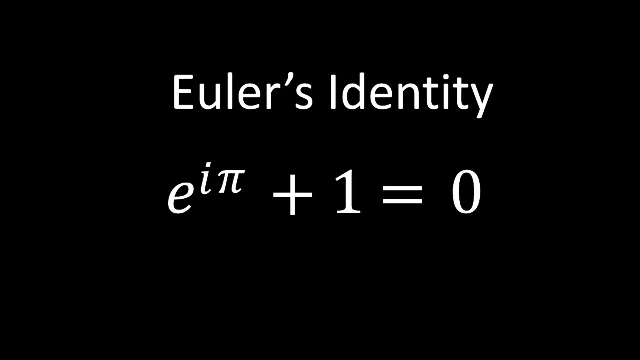 there are volumes of mathematics that Euler wrote that are still in use today. One of the things that he came up with- my personal favorite- is called Euler's identity, And Euler's identity says that e to the i, pi plus one is equal to zero. 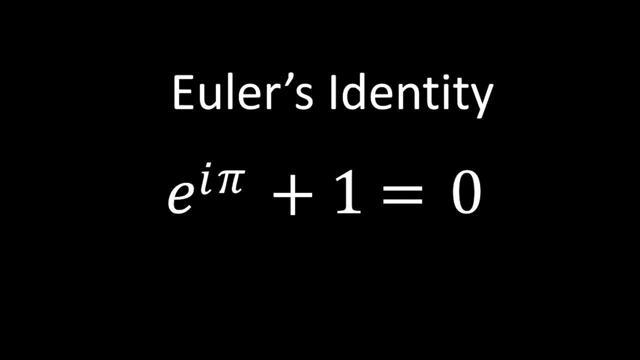 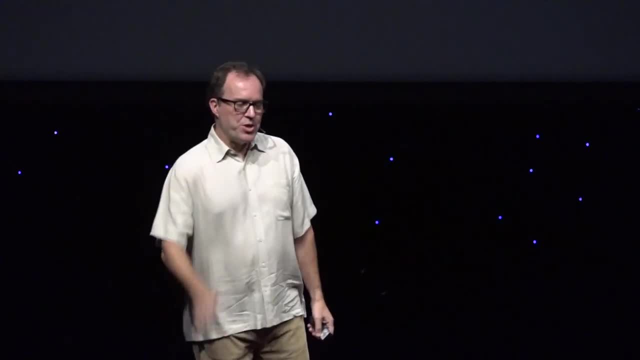 Now to the untrained eye this looks like a big jumble of numbers and letters and things like that. But if you give me a moment, I would like to train your eye a little bit. There are five numbers inside of Euler's identity. The first two that we 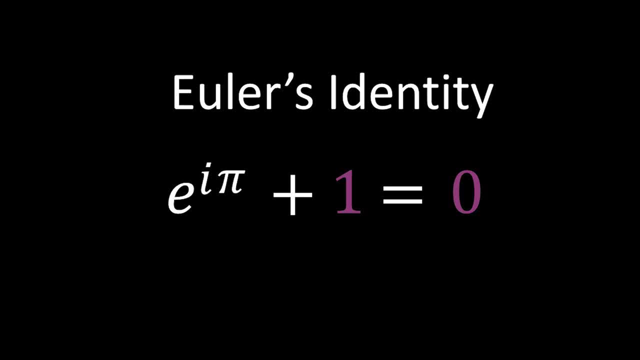 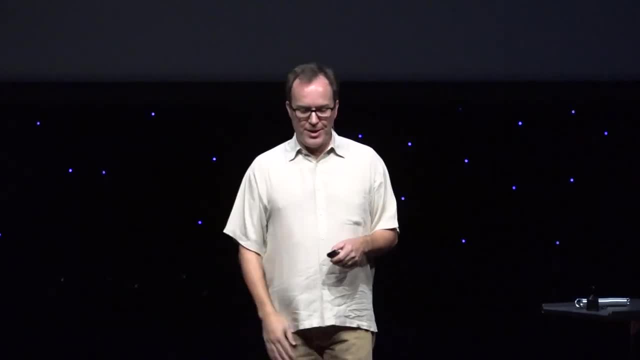 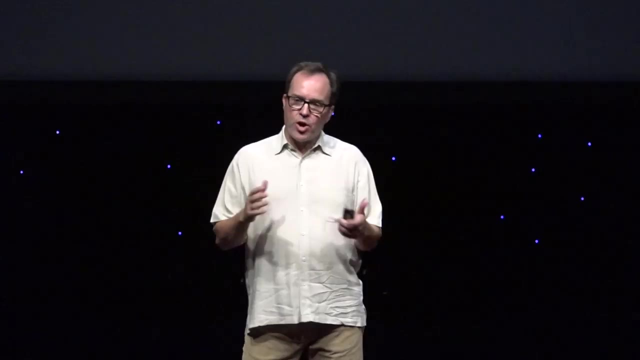 should look at are one and zero. These are real numbers And, without a doubt, they are the most important real numbers that we have. The next two that are in here are e and pi. These are real numbers. They can be plotted on the real number line. They are what we call. 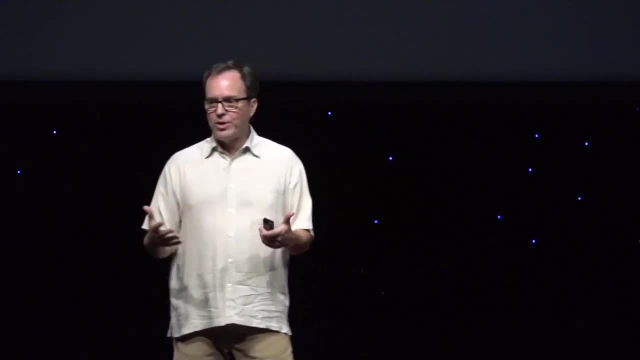 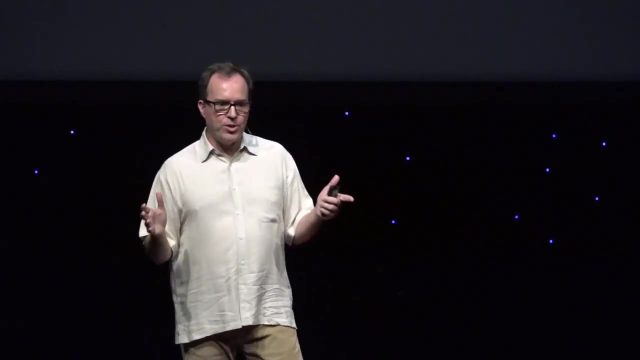 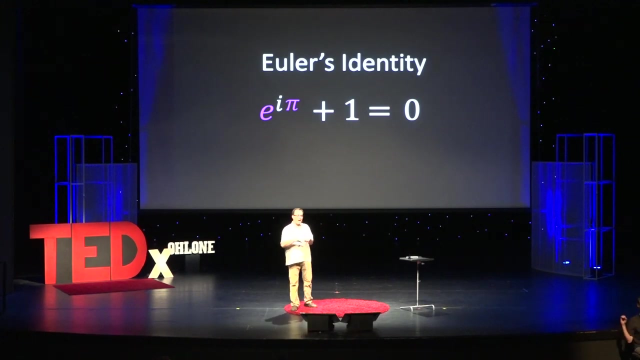 irrational numbers. Irrational numbers are real numbers that cannot be represented by a fraction. There is a vastly infinite number of irrational numbers, And e and pi are the two real numbers. There are two most important irrational numbers, And what is it that ties all of? 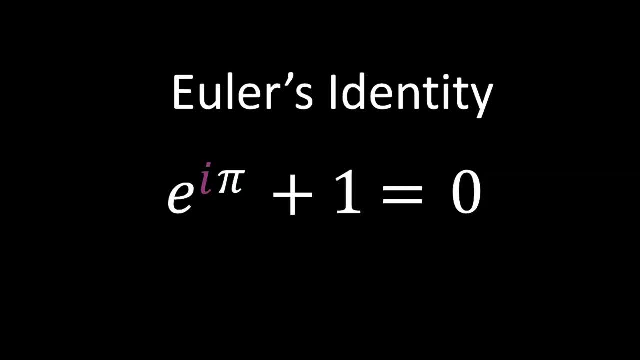 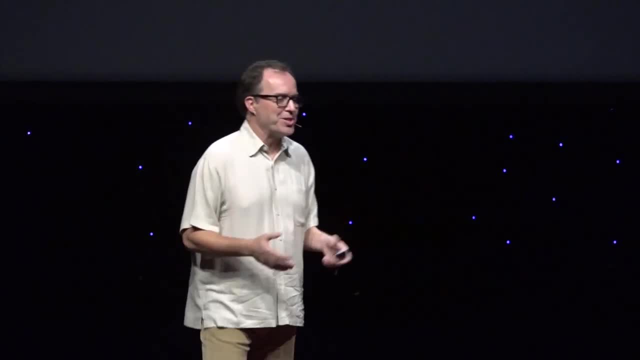 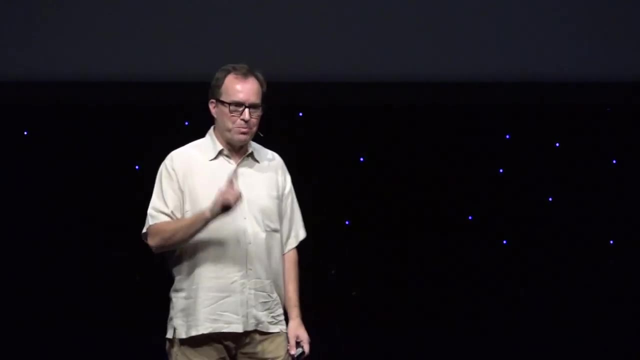 these things together. It's our new friend, the imaginary number i. This is called Euler's identity. There is a great social science experiment that is done on mathematicians and scientists on a fairly regular basis, where they are asked a simple question: What is the most beautiful equation? Yes, we tend to think. 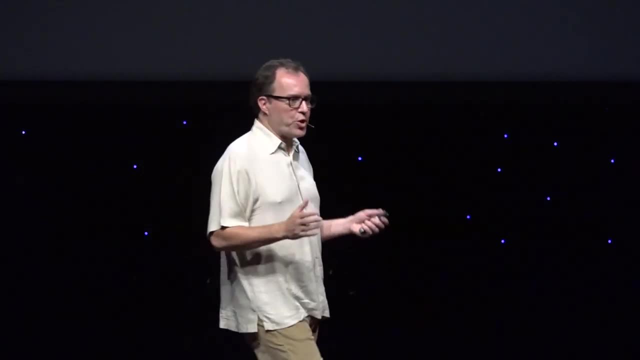 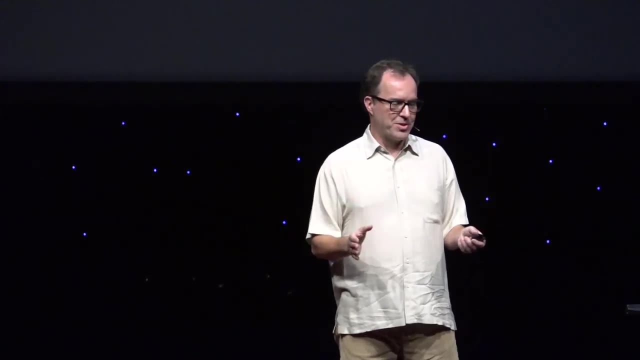 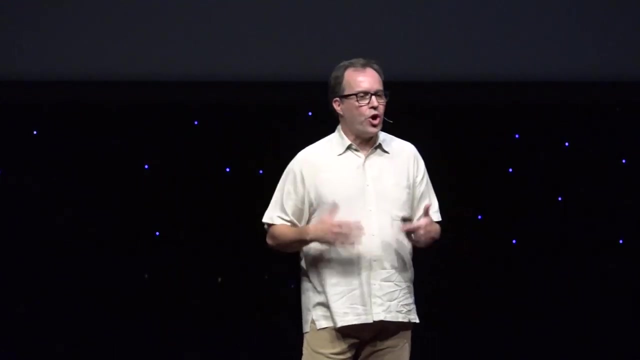 that equations can be beautiful. What is the most beautiful equation? Euler's identity often comes out on top or near the top of those kinds of surveys. So as I leave you tonight, it is my hope that when you are driving home and your car 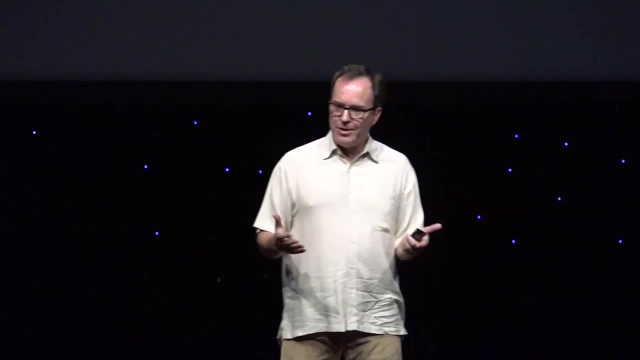 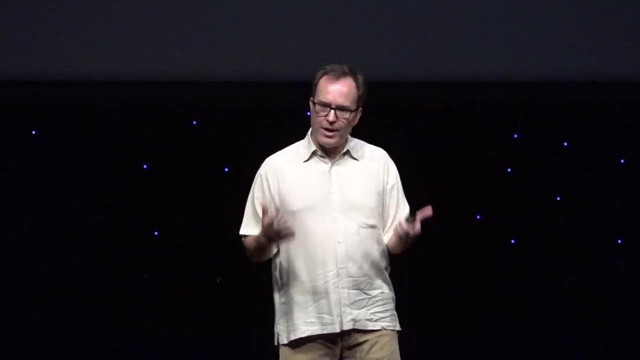 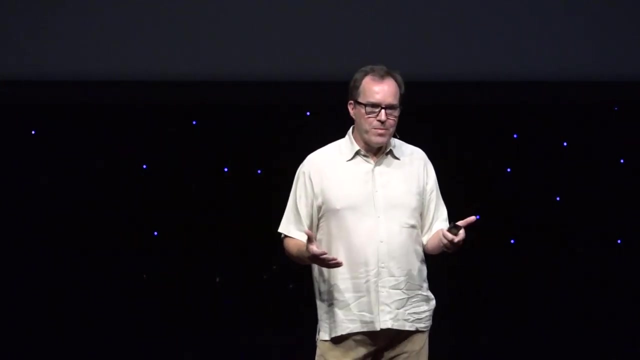 goes over a bump and the suspension system gently and quickly brings you back to a smooth ride. I hope you remember that complex numbers are not something that your algebra teacher invented to make your life miserable And, more importantly, I hope that you always remember that imaginary numbers are not imaginary. Thank you.